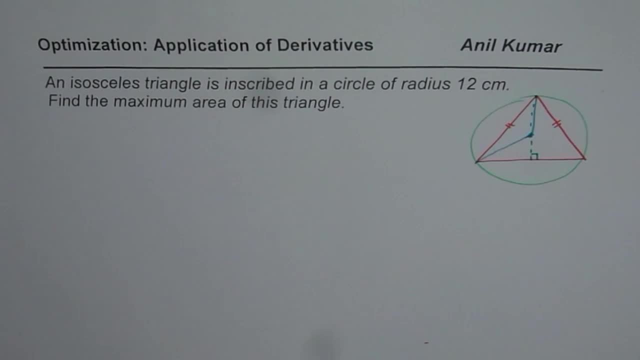 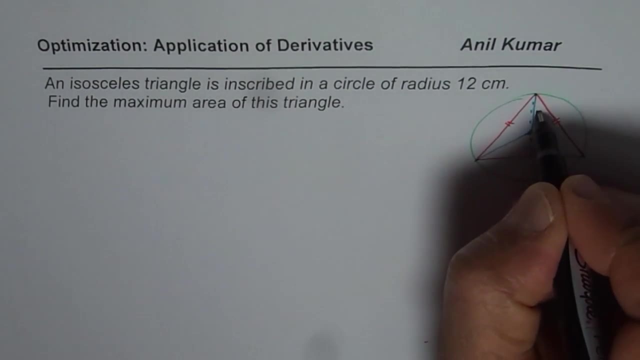 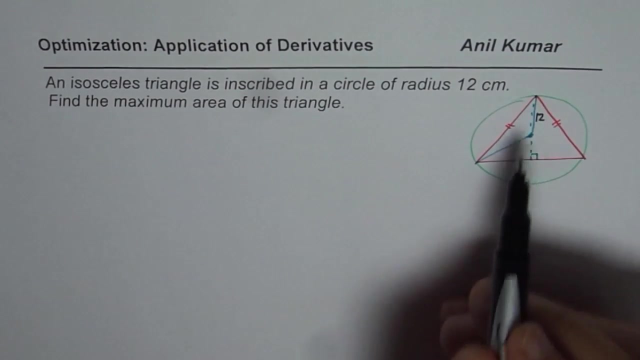 So what we are given here is that the radius of this circle is 12, and that gives you this side, which is 12. right, This is 12 for you. Now we need to find maximum area of inscribed triangle. Triangle inscribed in a circle. How to go about? 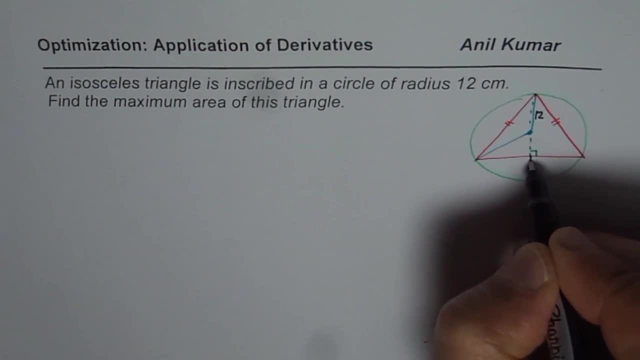 Okay, let us think that this side of the triangle is x and this is also x, and let us take this from the center to this end as y. Now, in that case, how are x and y related? So, in this small triangle, let me say this point is O. Let me label it be easy for us to discuss A, B, C. Let's call this. 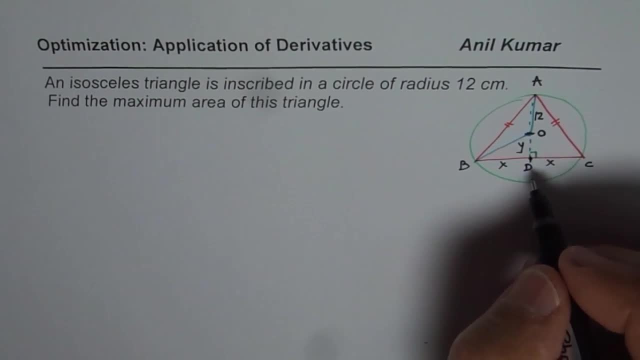 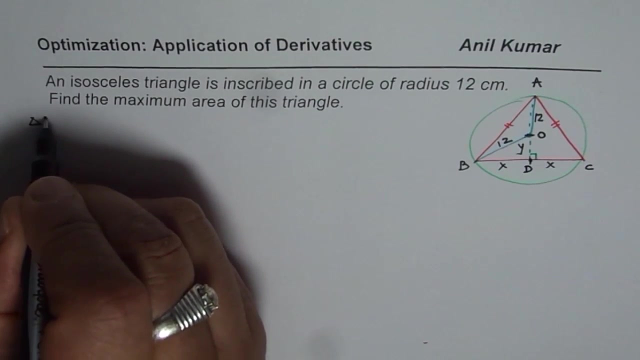 point as D, In that case O, D, which is y for us. Okay, so the radius over here is x and y for us. now give y this emergencies and suppose that we imagine that what we obtain from this triangle, we get the second action, we would get x角 plus y gratitude, already equal to 12, and once we 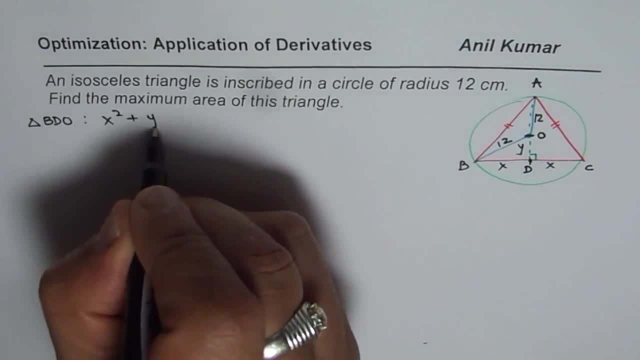 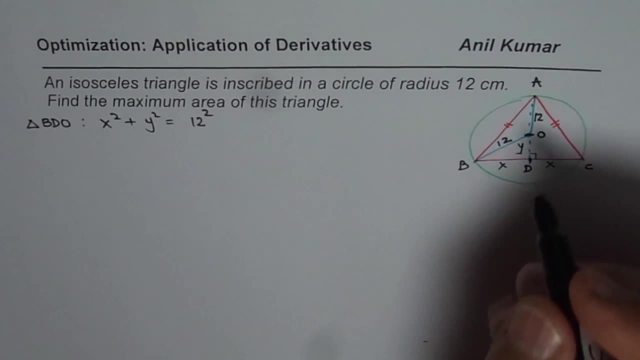 get y in that section. that's it. So we stripe it right and we get x in the middle and the pulls of the могу here in addition onto the red circle. we get that. we also get a lag, which we call x measure, fall of the angle, because one is. equal to the other and x. well, this dimension is the radius is also 12. so from the triangle, let us say bd- Let me write this as bdo- which is a right angle triangle, we know that x2 plus y2 equals to 12 squared. so that is what we got. This is one equation. 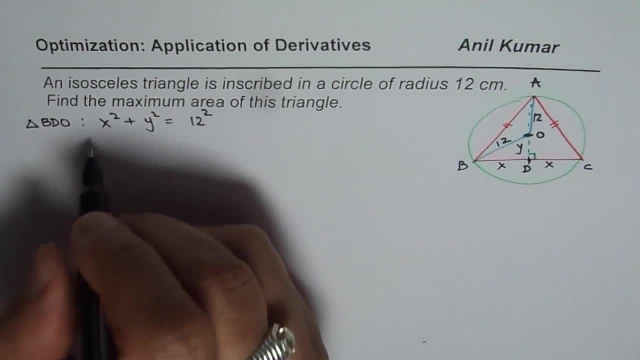 Now, from here, we can write one equation. One equation is this: we would be able to respond as products, when there is no detail, can write what x is. so we can write what x is. so we can say: x is equals to 12, square is 144. 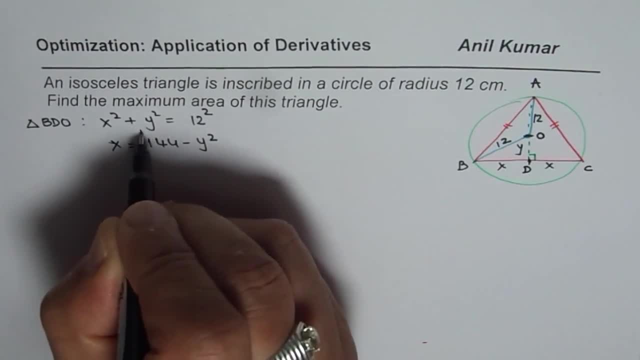 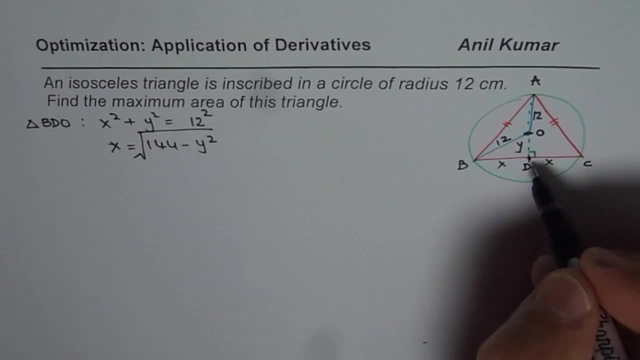 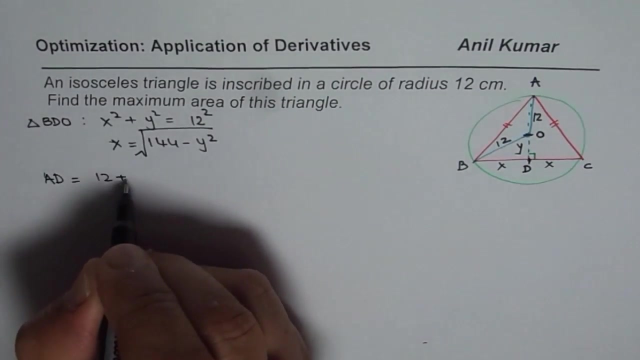 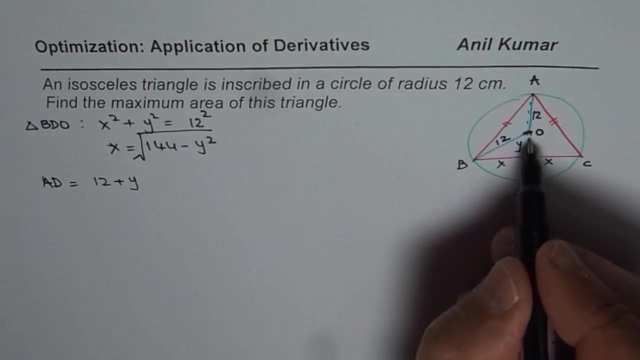 144 minus y, square square root. so that is what x is. now let us find the height of the triangle, which is ad. so ad will be equals to 12 plus y. 12 plus this is od is y. okay, perfect, now, knowing x and y, we can write down area of triangles. so we'll write area of triangle. 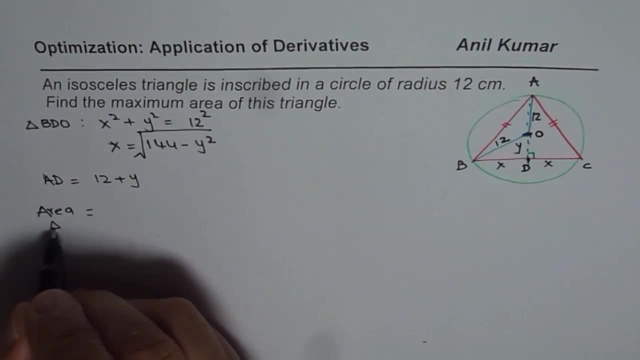 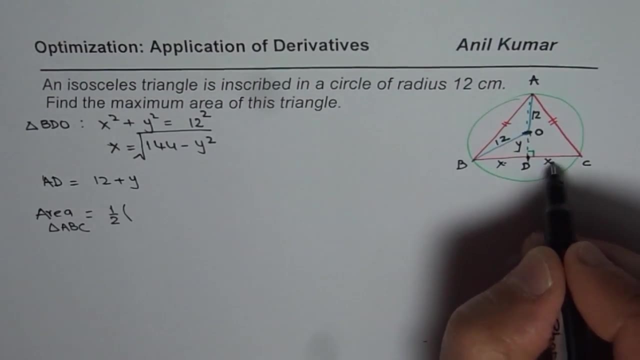 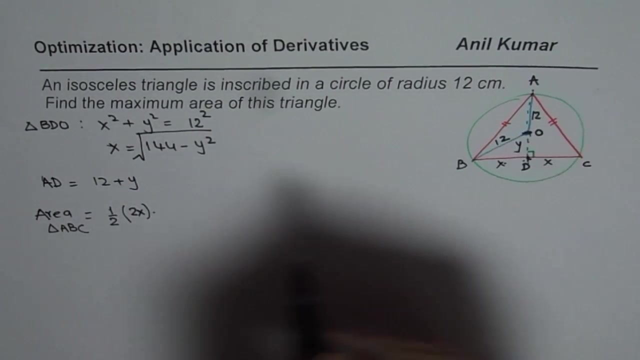 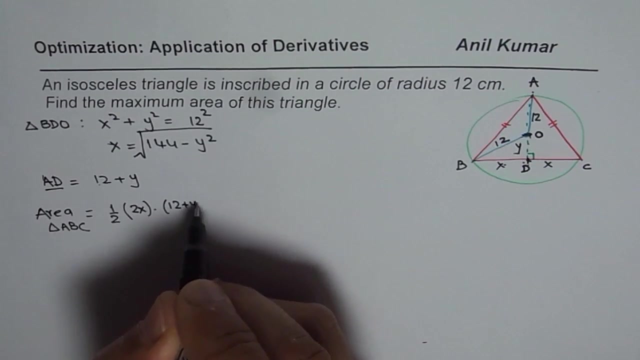 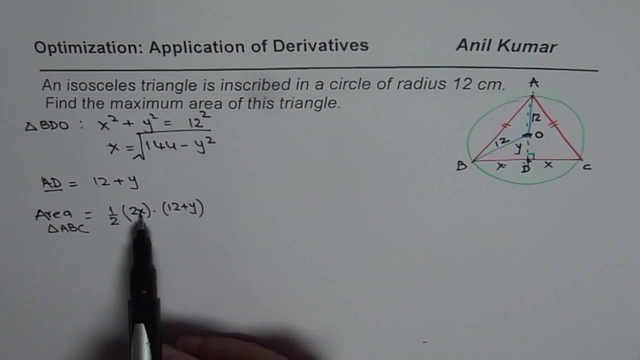 uh is equals to triangle a, b, c. we are saying right. so triangle a, b, c, half base, half of base, is two times x, correct? 2x. half base into height, which is ad, and this height ad could be written as 12 plus y. so half base into 12 plus y. so that is how we get the area equation. now second step is we need to 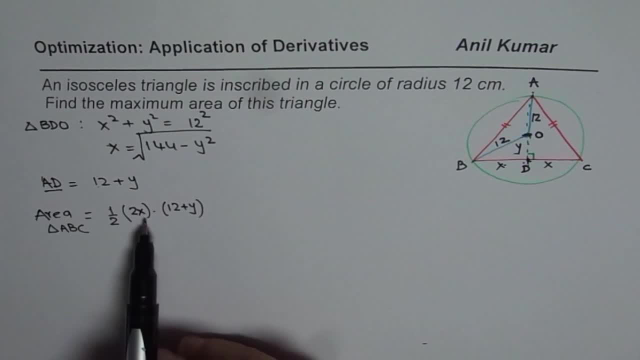 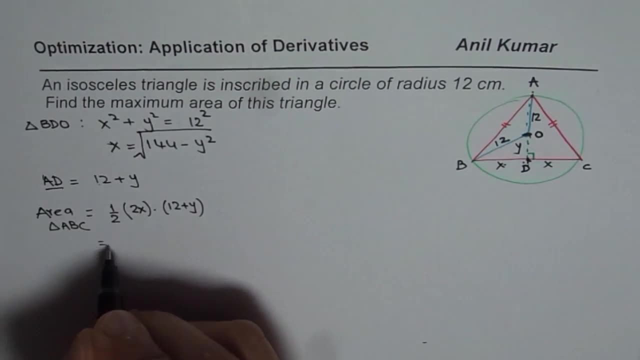 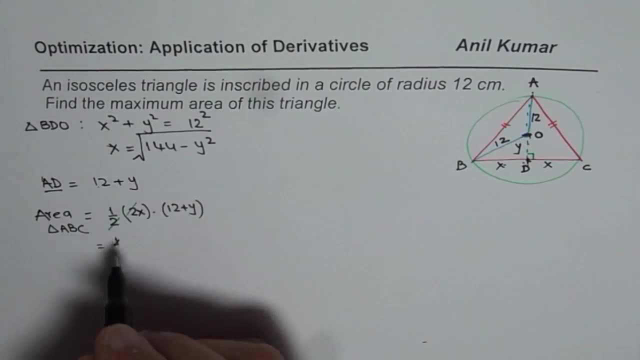 write this equation in one variable. so i'll replace x with that square root function. okay, so that is how we could replace x with: so we get this equation as half and two cancel out. okay, that's good. so let's cancel this out. so we have x times 12 plus y, and x is equal to 144 minus y square. so we'll write this as: 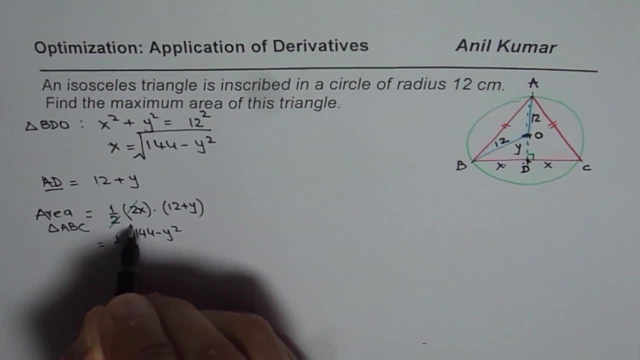 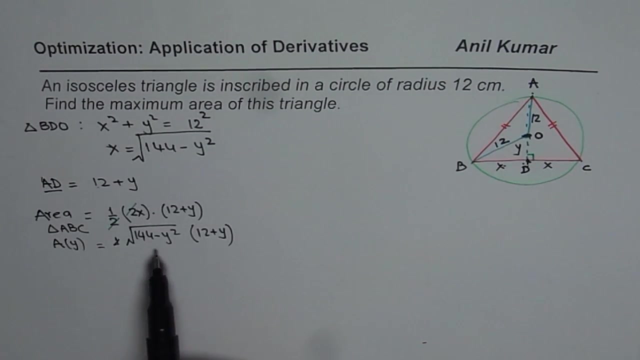 square root of 144 minus y, square times 12 plus y. so that is the area, and all this area is in terms of y. so i'll write area as a function of y. perfect to maximize. what can we do to maximize? we can find the derivative and find critical number right. so let's find the derivative for. 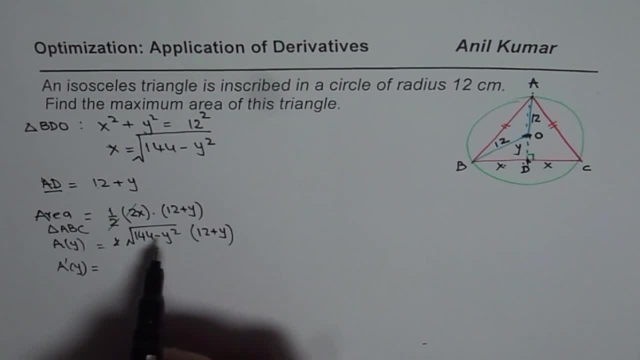 this function, which is apply the product rule derivative of the square root part, is one over two square root of 144 minus y. square times: minus 2y right, minus 2y, minus 2 y. So let me write this: minus 2, make this as y. okay, minus 2 y. So that is the. 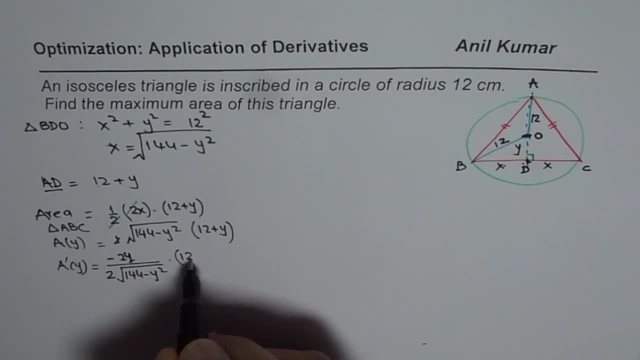 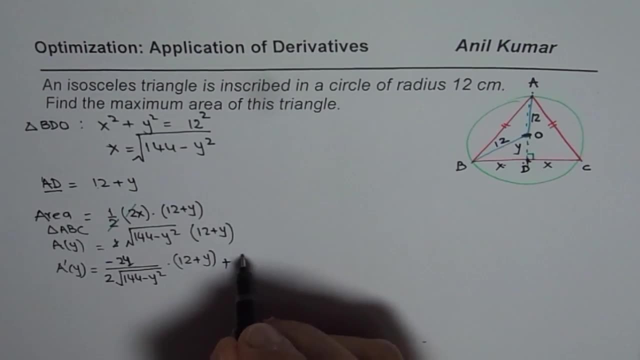 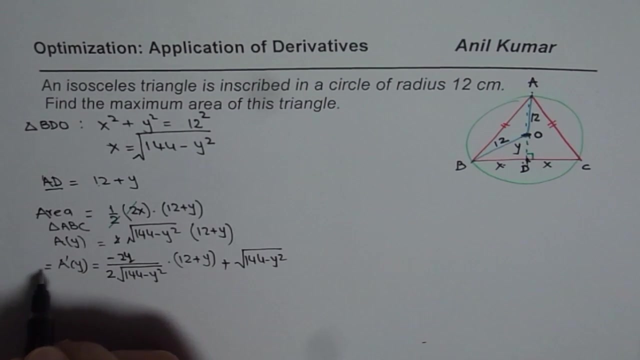 derivative of this function times 12 plus y plus derivative of this function is 1 times this, which is square root of 144 minus y square. So that becomes the derivative. We can equate this derivative to 0 to find the critical number. So this I have done to find critical number. Great. 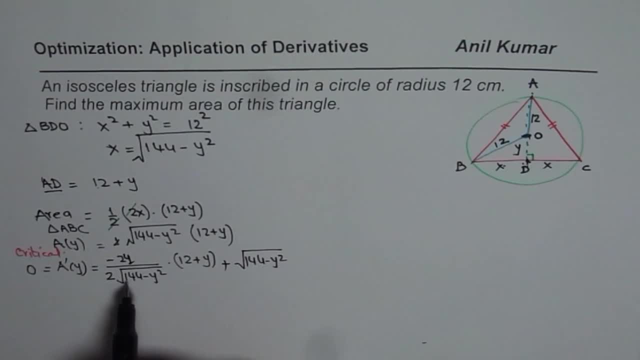 Now. so what we can do now is multiply by the 2 and 2 cancers, again multiply by the square root term. So if I multiply by square root term, then we can actually simplify it more, right. So what we will do now? first let us multiply and say 0 equals 2.. 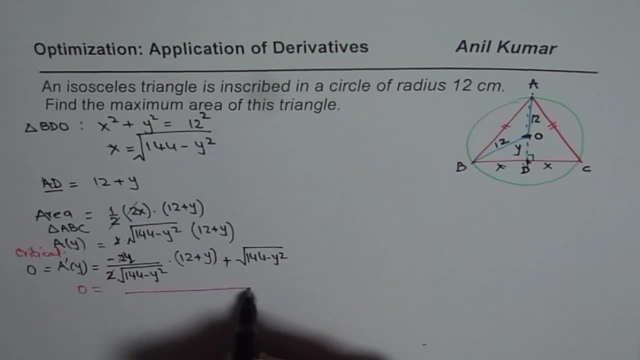 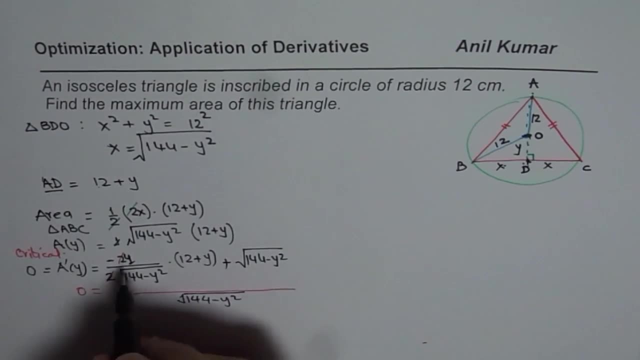 So if I or we can take common denominator, it is one and the same thing. So we will take common denominator 144 minus y square. Here we have minus y times this, So we have minus y times 12 plus y, and when you multiply this the square root goes. So we get plus 144 minus y square. 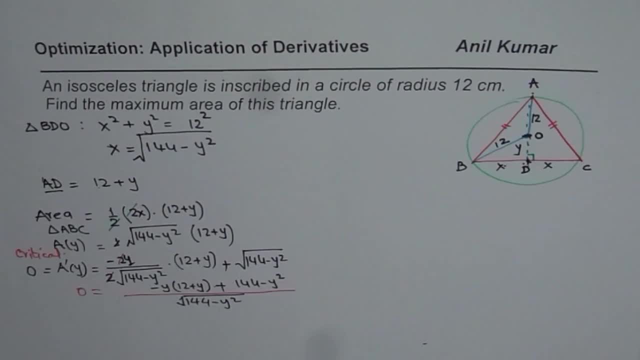 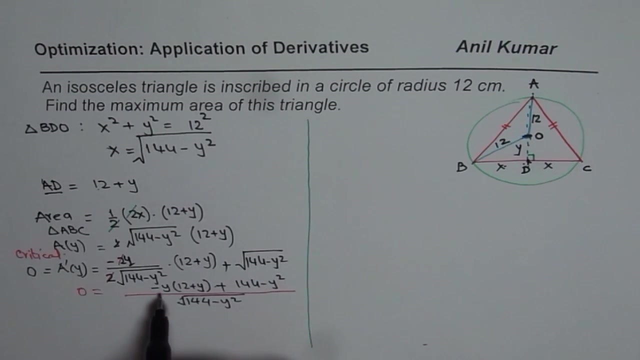 Do you see that? So that is what we get. So we can simplify the derivative to get the critical numbers. So this can be 0 if the numerator is 0, right, So what we have here is numerator which is equal to 144 minus y square, and here we have minus y, 12 plus y. 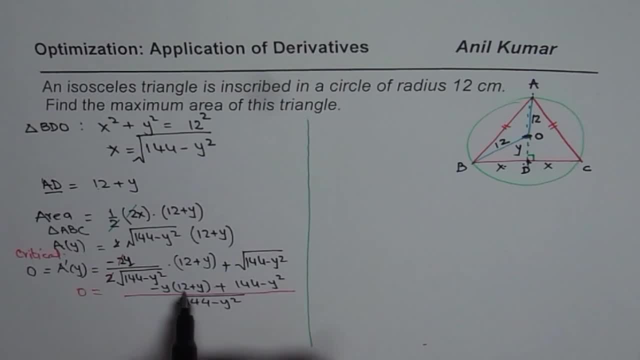 You see, this is like 12 square minus y square, So 12 plus y is a common factor, right? So that is kind of a tricky part. So what we want to do here is we want to write this as see: this is 0 equals 2.. 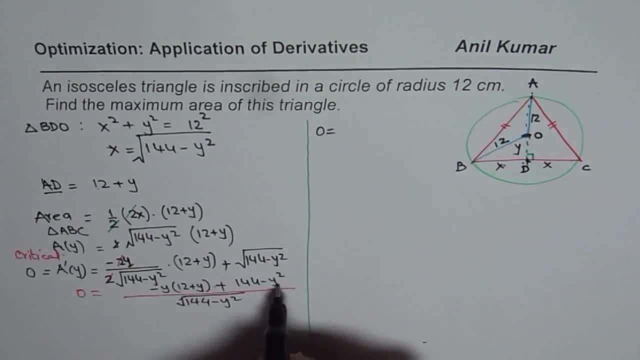 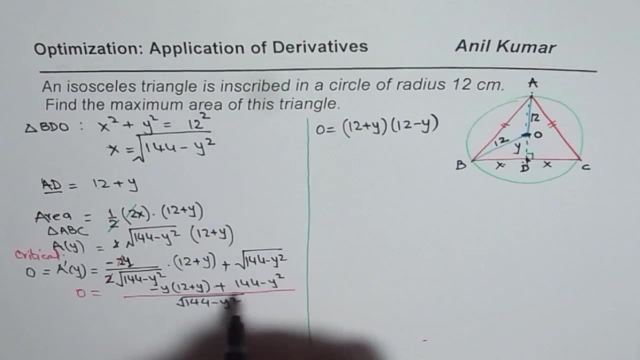 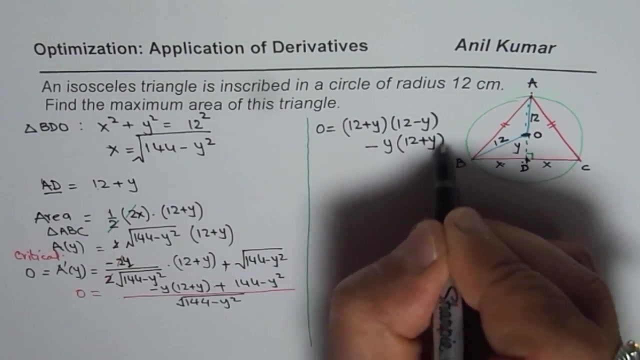 Let me write this as 144 minus y. square could be written as 12 plus y minus 12 minus y, right? So that is this part, correct, minus that part which is y times 12 plus y. You get the idea. 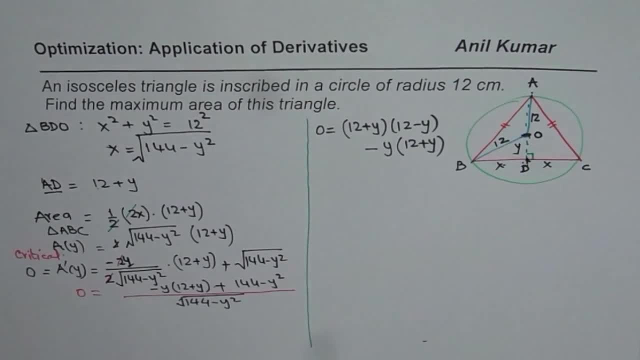 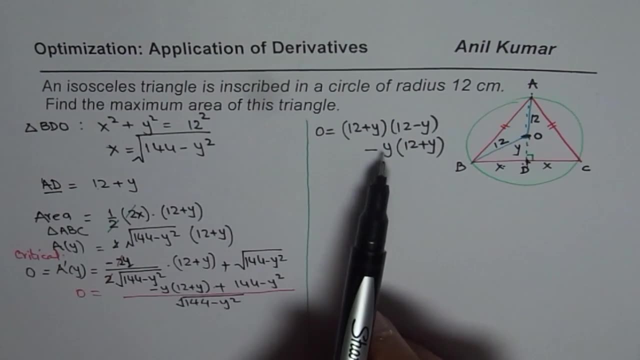 So the numerator can be written. this, So the denominator can be written in factor form. This is a very critical step to understand. It helps to find the critical number. You could actually expand and then also do That is also equally good. Minus y square, minus y square will cancel and you will easily find the value also correct. 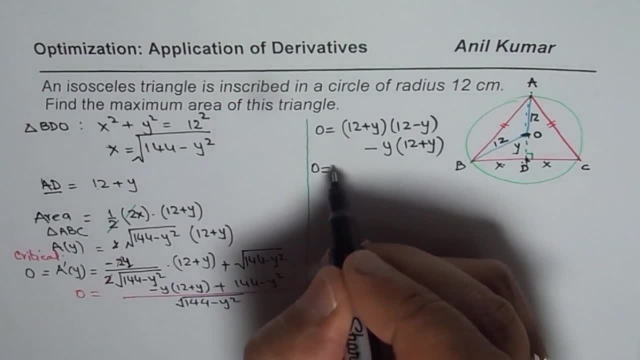 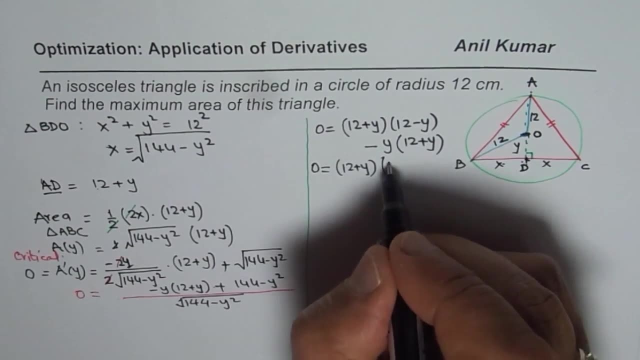 Anyway, I prefer to do factoring here. So 12 plus y is common factor. So we are left with 12 minus y, And here we get minus y, right. So 12 plus y and 12 plus y is a common factor. 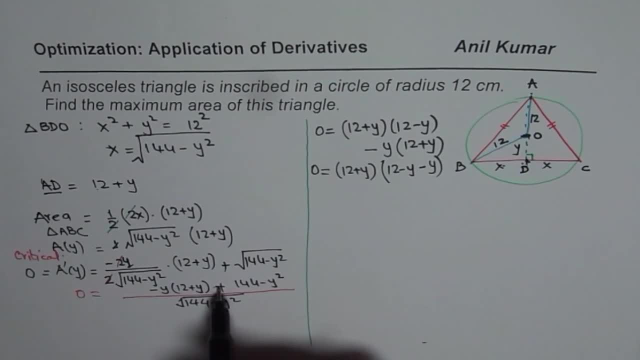 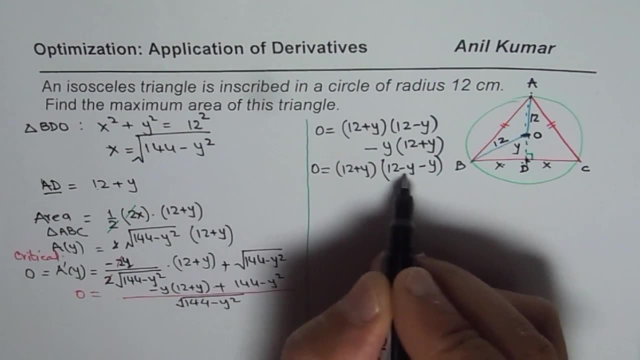 So we are left with 12 minus y. Now these are 0, for y equals to minus 12, but y cannot be 0. Y cannot be negative, but this gives us a value of 6, right Minus y, minus y. 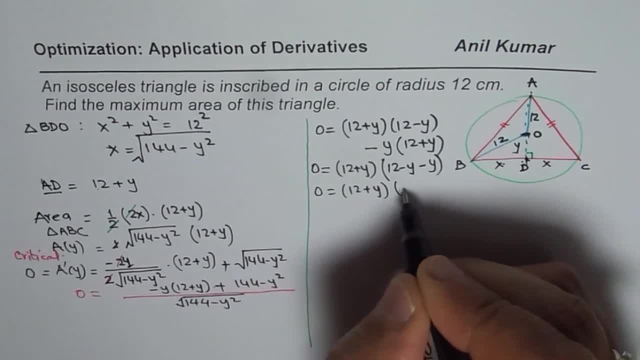 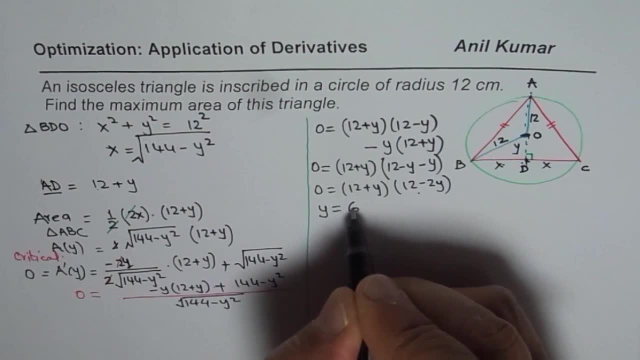 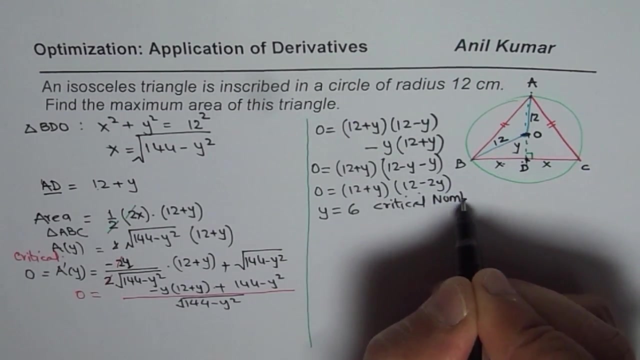 So this is right as 12 plus y Y times 12 minus 2y, So that is 0, for y equals to 6.. So y equals to 6, is our critical number, Perfect. Well, you could have expanded and got that easy, No problem. 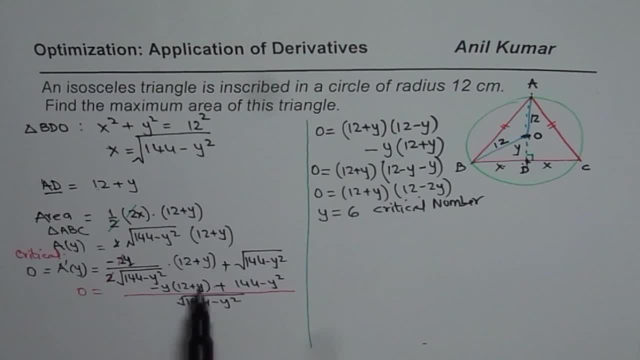 So you could have easily done it. When you square y times y, they cancel out. Minus 12y equals to 144.. And you get your answer, Which is Okay. so the critical number is y equals to 6.. 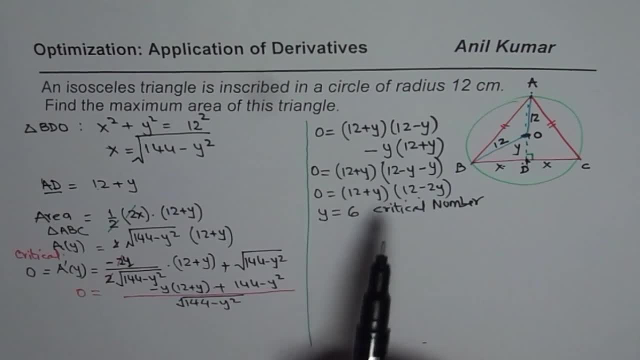 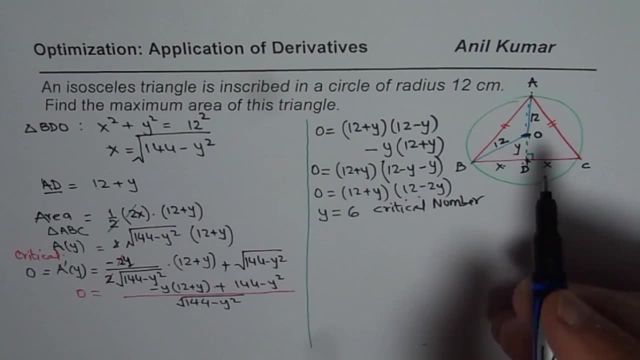 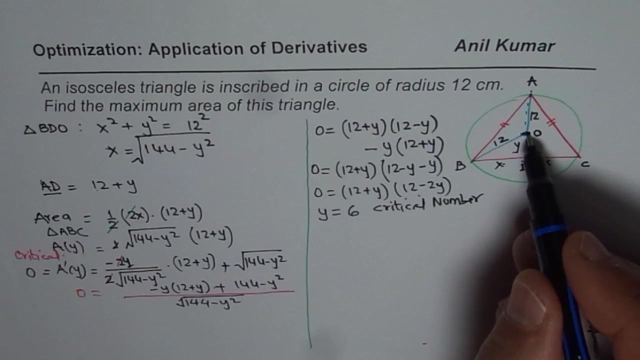 We need to now show that for y equals to 6,, the area is indeed maximum. Now there are a couple of ways to do this from here. What we can do is we can see what is the limit of the y value. y could be from 0 to 12, because it is within the circle. 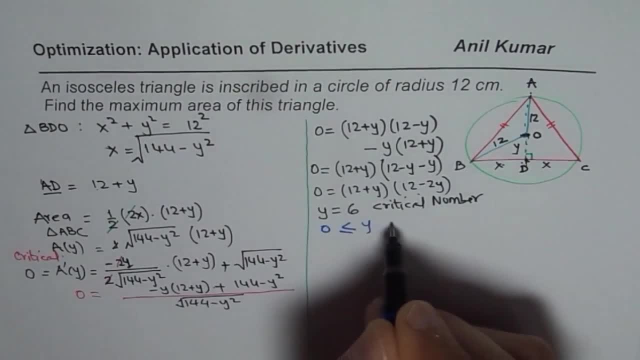 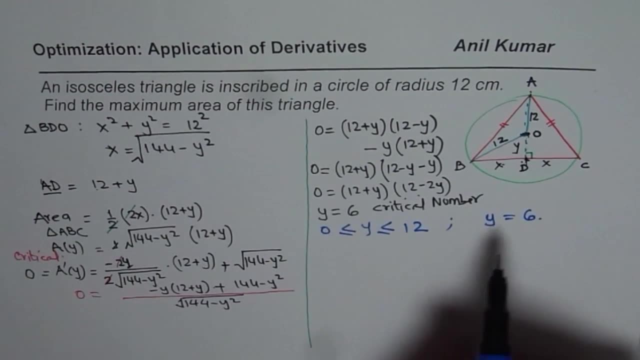 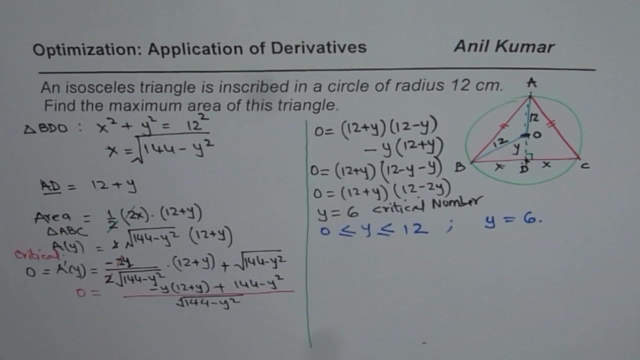 So we have a boundary condition here which is y is between 0 to 12.. So that is the boundary condition and our critical number is: y equals to 6.. So we need to test the value of area with these three values, So we will find the area which for us is integral. 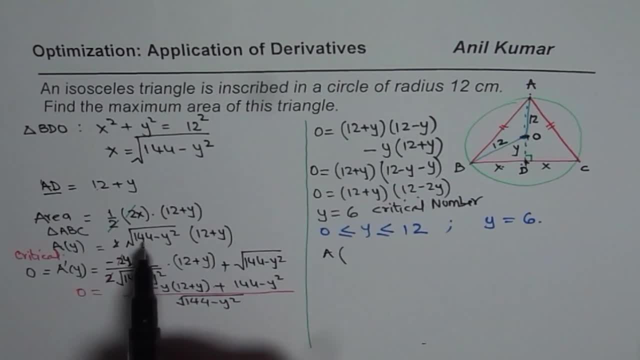 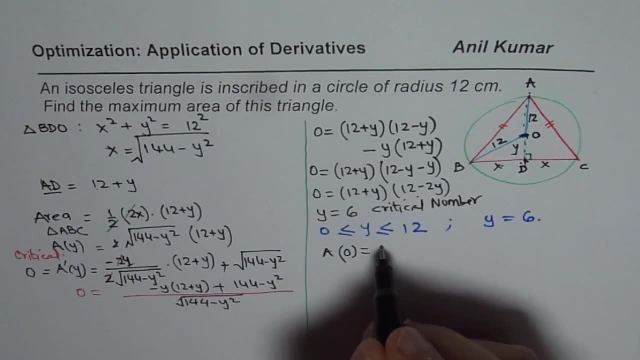 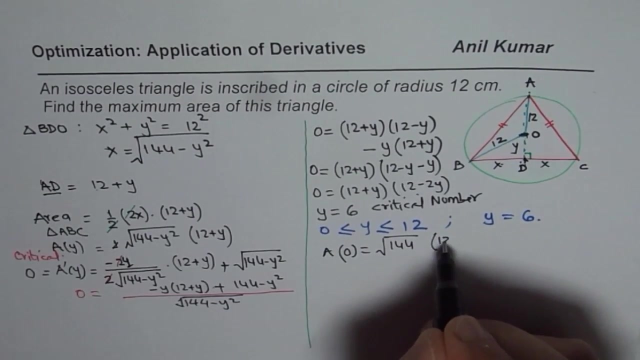 In terms of y written here half base into y. we got this formula So area for 0, if I write y as 0 in this area, what do I get? I get square root of 144 minus y, square 0 times times 12.. 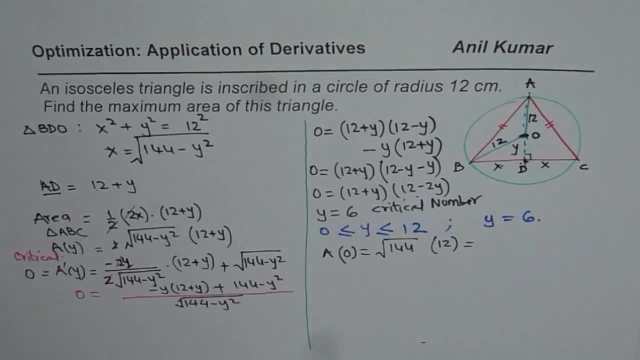 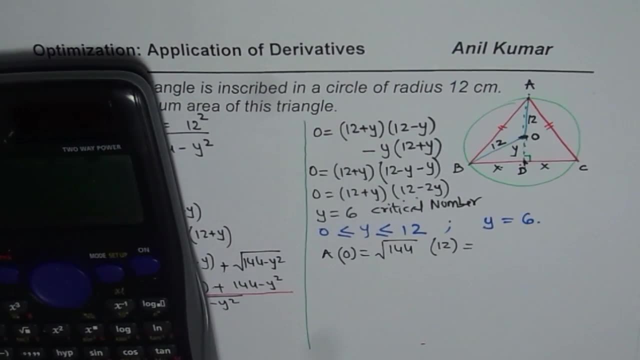 So that is 1.. If I write so, let us use this value. We know square root of 144 is 12,. 12 times 12 is 144.. Anyway, let us calculate. So square root of 144 is equal to 12 times 12 is also 144.. 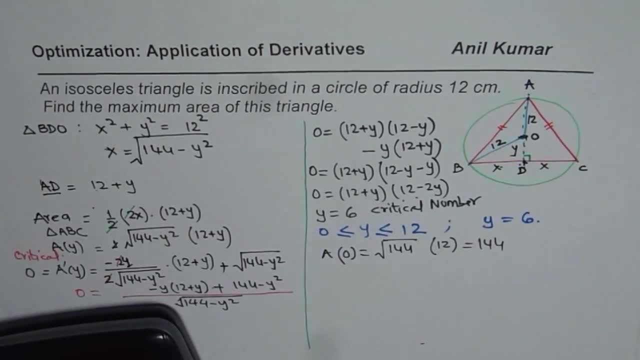 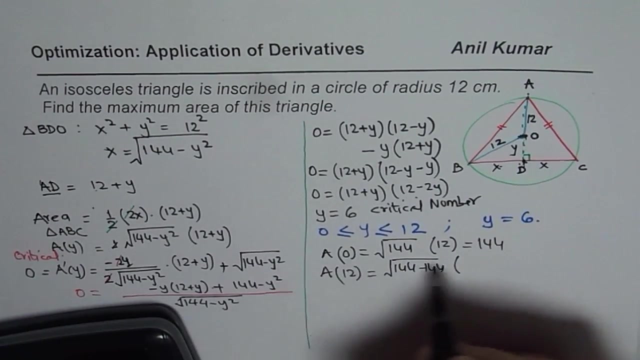 This is 144.. Similarly, let us find area for 12.. So if I write 12 here, so I get square root of 144 minus 144 times 12 plus 12.. Now 12 plus 12 is 24.. 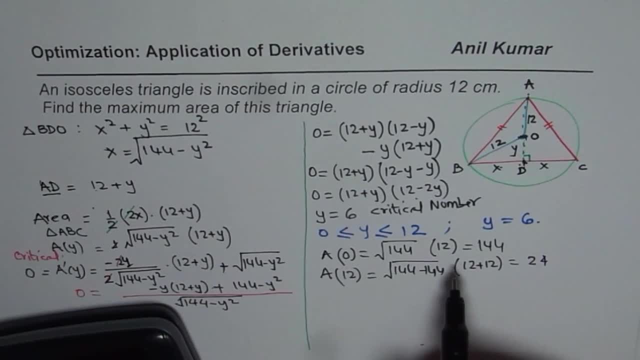 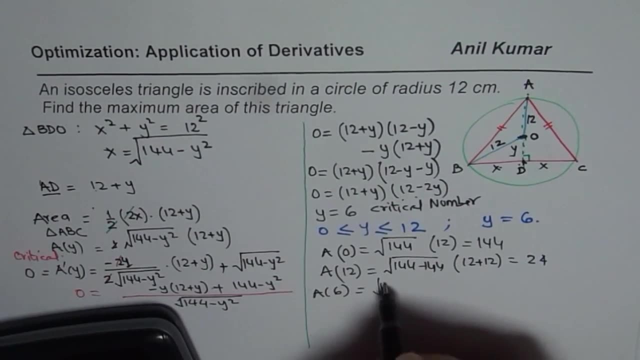 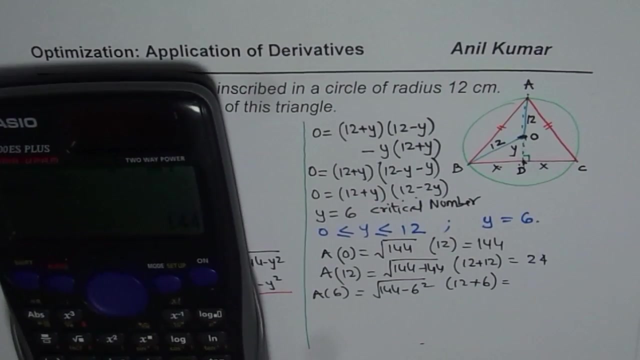 So we get 24 this time. Now, that is 1.. The third is for 6.. So let us find area when y is 6.. So we have square root of 144 minus 6. square times 12 plus 6 equals to how much? 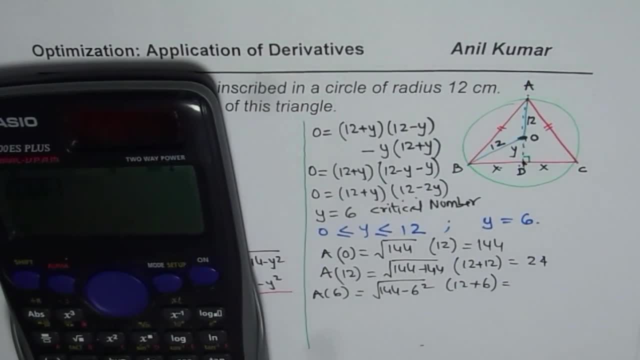 So we have square root of 144 minus 6 square, which is equal to 6 square root 3.. We will multiply this by 12 plus 6, which is 18.. And that gives us 187.06.. So, comparing these values, what do we find? 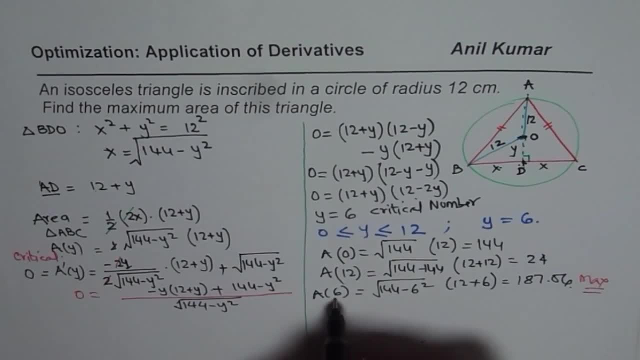 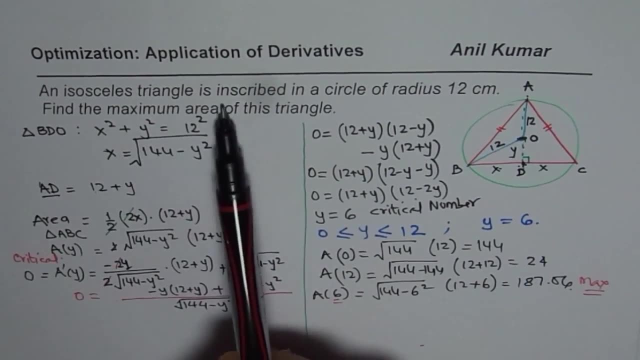 The maximum is for y equals to 6.. So maximum is for y equals to 6.. Now the question is: an isosceles triangle is inscribed in a circle of radius 12 centimeters. Find the maximum area of this triangle. 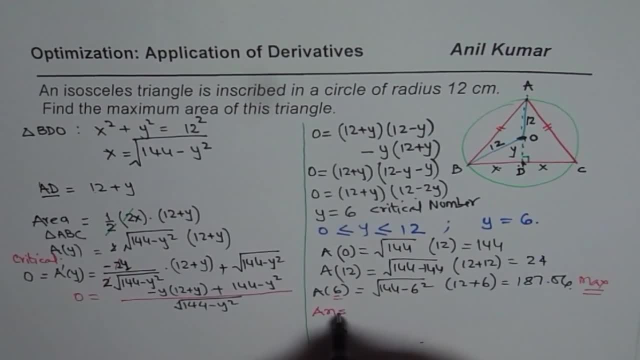 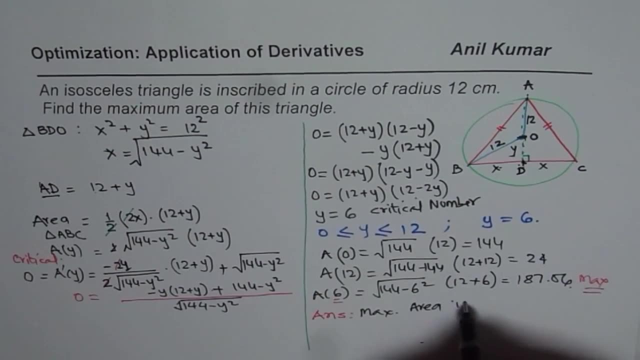 Correct. So you have to read the questions so that you can exactly answer. So the answer here is: maximum area should be 187 and the units are centimeters squared Right, So approximately 187 centimeters squared. I hope with this the steps are absolutely clear. 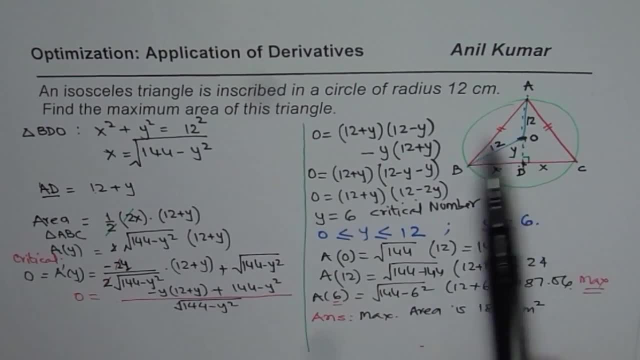 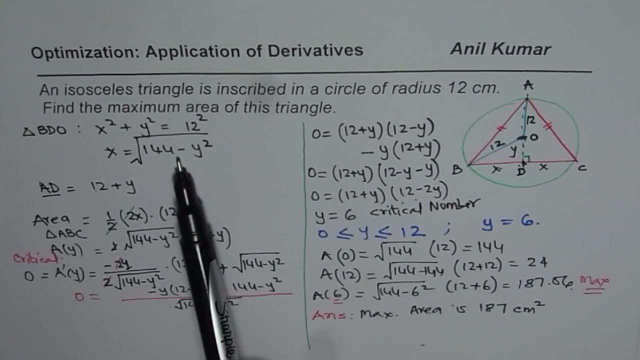 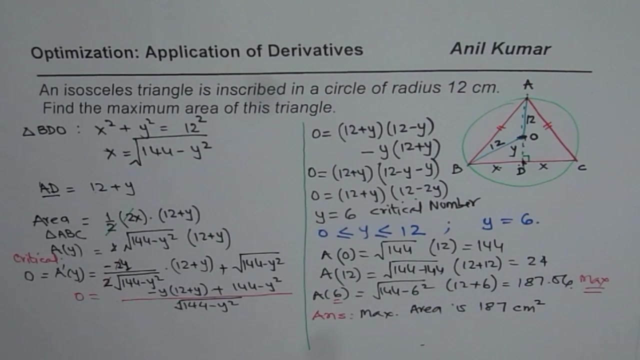 So first sketch to represent the situation, define your variables, relate the variables so that you could write 1 in terms of the area- Okay- And then write the expression for the area, find the derivative critical number, boundary conditions, and then get your answer.